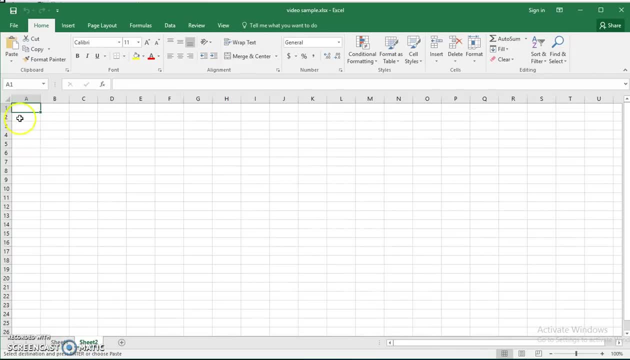 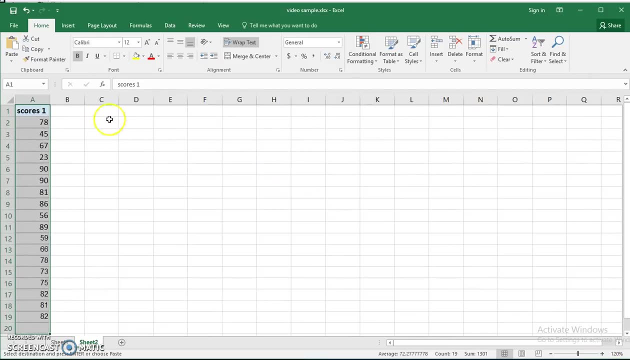 So first of all, I'm going to copy it to a new worksheet So we don't have to be distracted by other things. Then I want to find out what is the highest number and the lowest number in this data, So I can set up my class limit properly. 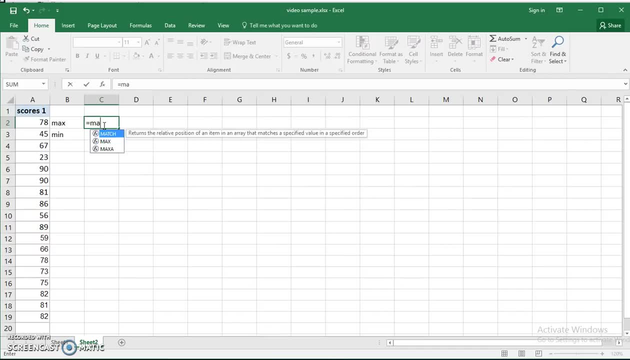 So Excel can do this by using a function called EqualMax. EqualMax- open parenthesis. you just give the data to it. Excel will look at it and tell you: oh, the maximum is 90. And then EqualMin- the data value: the lowest is 23.. 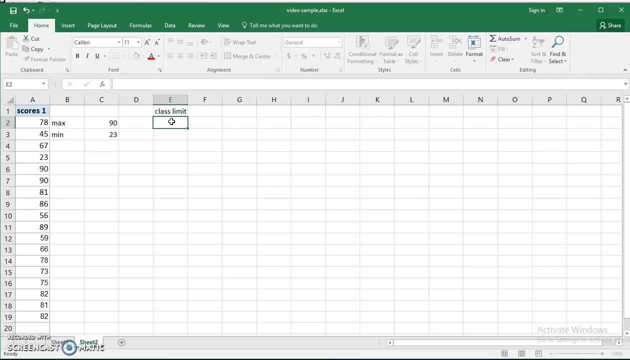 So our logical class limit would be: you know, need to include 23.. So the lowest should be around 21, and we wanted to start with a nice number instead of starting from 23.. So 21 to 30 seems to be a nice class limit to go with. 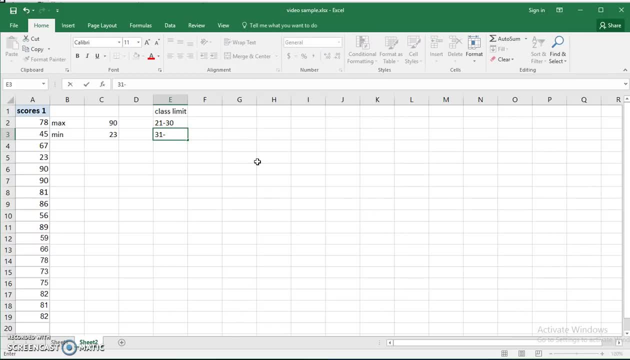 And then I do 31.. So 31 to 40,, 41 to 50,, 51 to 60,, 61 to 70,, 71 to 80,, 81 to 90.. So you have to create this, you know, based on whatever data that you have. 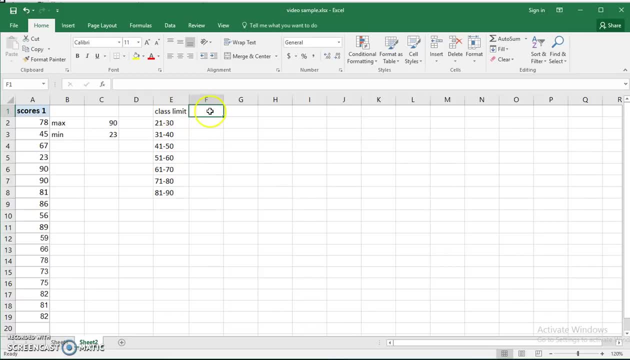 Now, but Excel, do not look at this. Excel wants a column. It contains only the upper class limit, So what you can do is just copy all the upper class limit in a separate column for Excel to use. The class limit is for us to use and also for us to build a table. 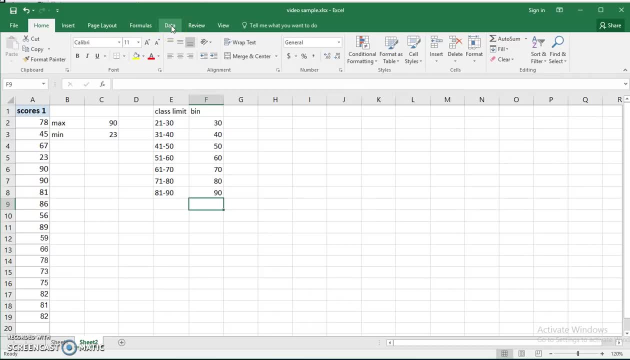 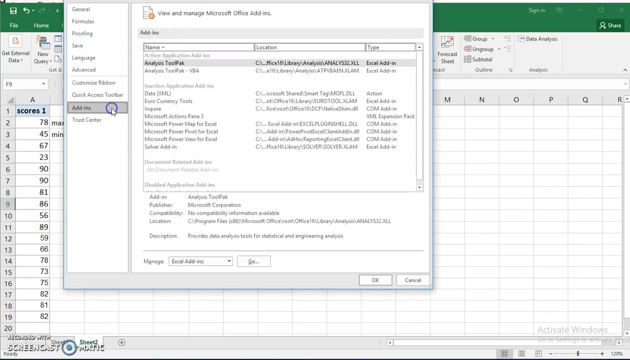 Now we are ready. So this and then to build them. So what you can do is click data and see if data analysis is here. If data analysis is not here, you go to file option Add-ins- manage Excel add-in. go and enable the first two. 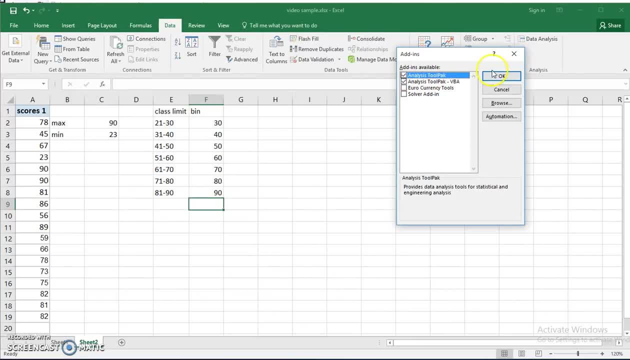 Or I think just the first one is fine- Check them and then say: okay, In my case I have data analysis available, so I don't have to do that, Or it has already been done, You only need to do it once. 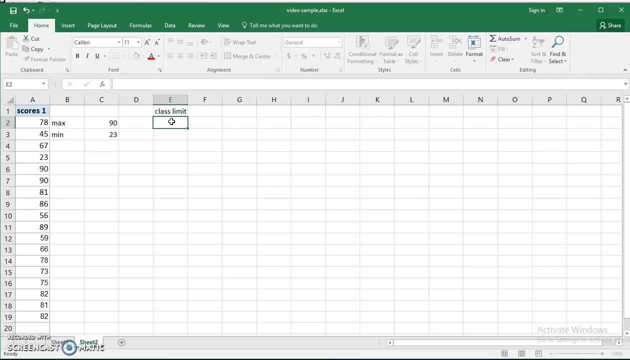 So our logical class limit would be: you know, need to include 23.. So the lowest should be around 21, and we wanted to start with a nice number instead of starting from 23.. So 21 to 30 seems to be a nice class limit to go with. 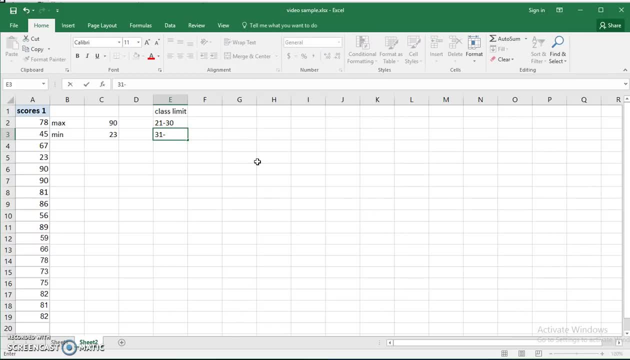 And then I do 31.. So 31 to 40,, 41 to 50,, 51 to 60,, 61 to 70,, 71 to 80,, 81 to 90.. So you have to create this, you know, based on whatever data that you have. 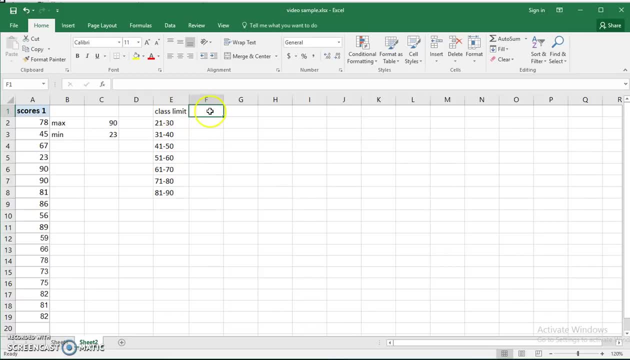 Now, but Excel, do not look at this. Excel wants a column. It contains only the upper class limit, So what you can do is just copy all the upper class limit in a separate column for Excel to use. The class limit is for us to use and also for us to build a table. 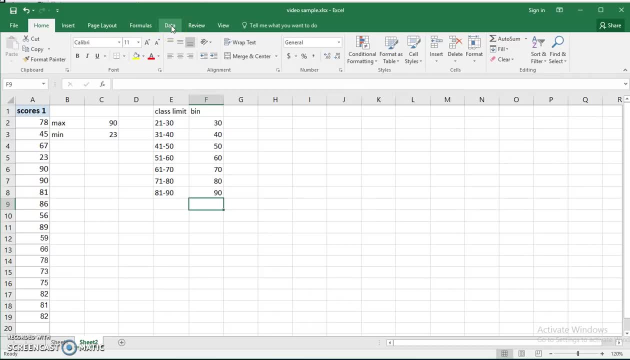 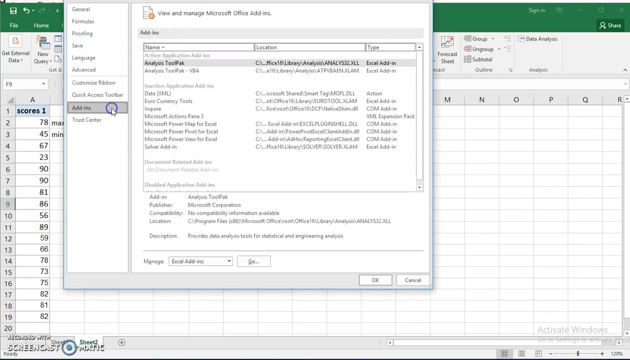 Now we are ready. So this and then to build them. So what you can do is click data and see if data analysis is here. If data analysis is not here, you go to file option Add-ins- manage Excel add-in. go and enable the first two. 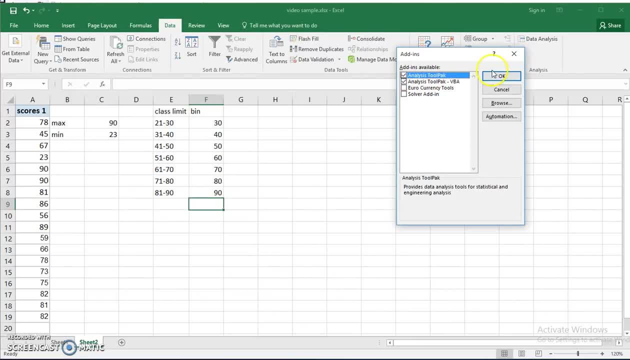 Or I think just the first one is fine- Check them and then say: okay, In my case I have data analysis available, so I don't have to do that, Or it has already been done, You only need to do it once. 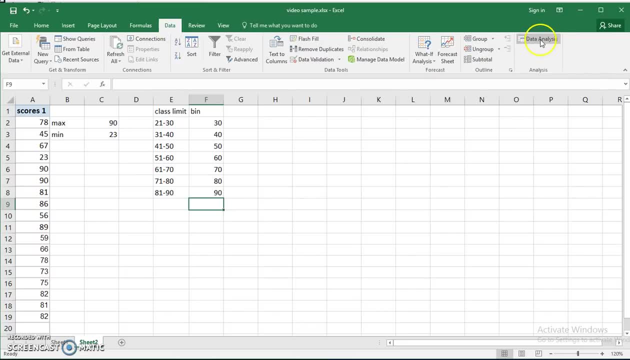 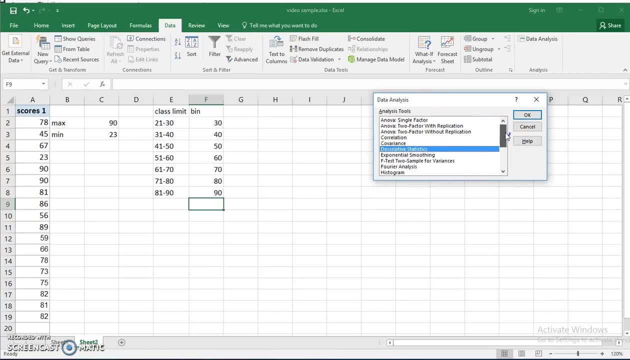 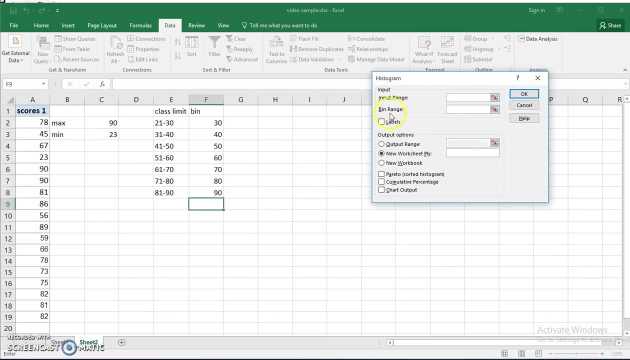 So you can see here. So you can see here Packages or modules available, and the one that we want is histogram And you click okay, The first thing you need to tell Excel is your input range, which is all your data, And in my case, I want to provide the header also. 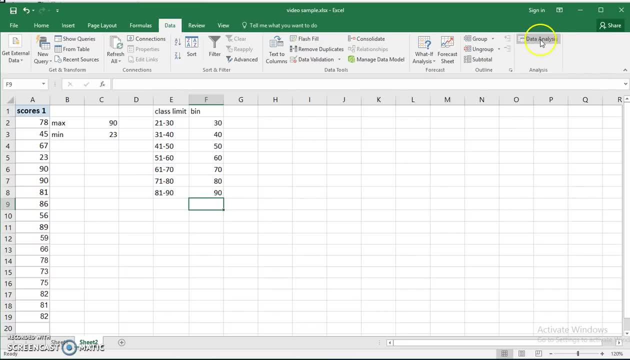 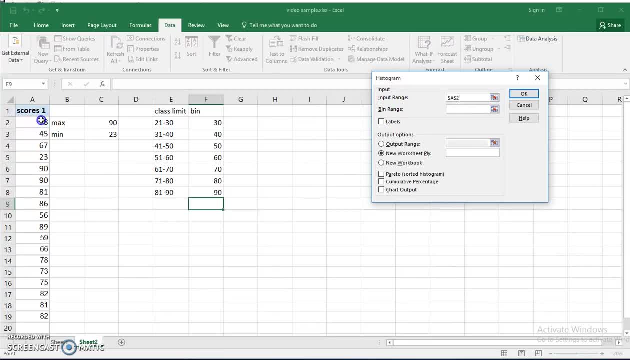 The first things you need to tell Excel is your input range, which is all your data, And in my case I want to provide the header also, So I click label. That means the first one is not a data value, but it's a label. 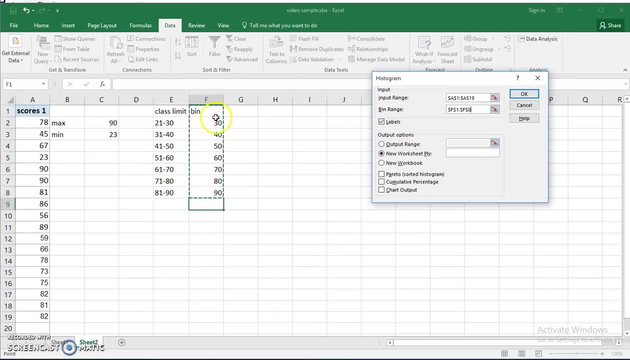 And then under bin range would be the upper class limit. So I include the bin header label also. then for the output option, I want Excel to just put the output in this worksheet, so I click a cell in the output range. the last thing I want to do is check output, so the histogram would show up, might say okay. 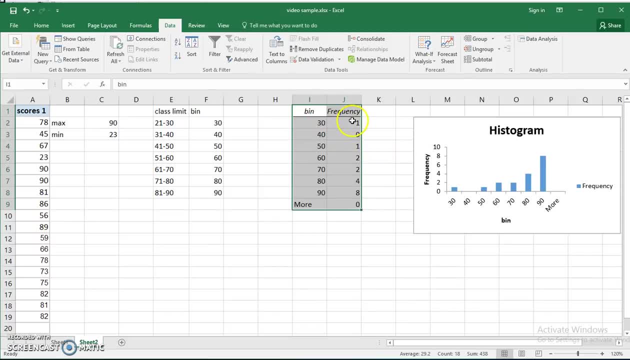 see, I would have. this is the frequency distribution for each class and also this is the histogram. we need to do some adjustment. first of all, we'll copy this over. well, actually, I just need to copy the frequency over in a new area face and use the what, the class limit that we have set up. 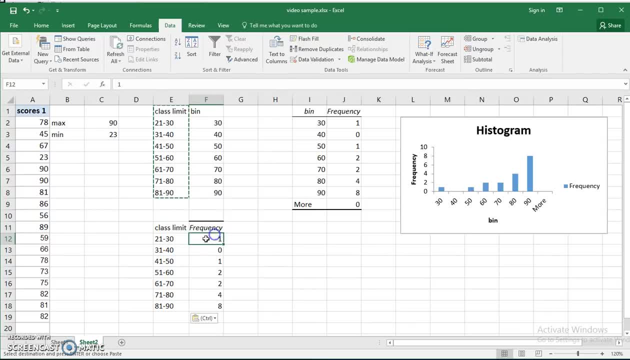 so they. this is the class, this is the frequency for this class, there's one data between 21 to 30 and there's a corresponding data values in this range, and that would be our frequency distribution. and you can, you know, make it nicer by putting in: 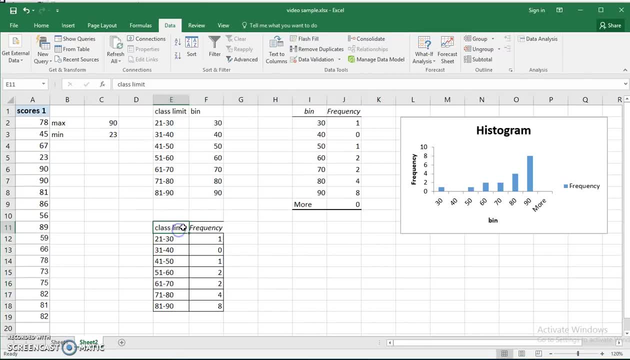 the borders. that's it, and maybe you want to change it. not instead of class limit, you want to say as scores for class one, something like that, and then for our histogram what we can do is change the title, so maybe you would say histogram for class one: frequency. instead of being it should be score. 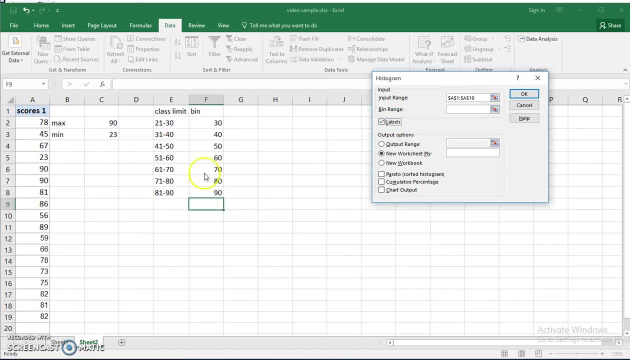 So I click label. That means the first one is not a data value but it's a label. And then under bin range would be the upper class limit. So I include the bin header label also. then for the output option, I want Excel to just put the. 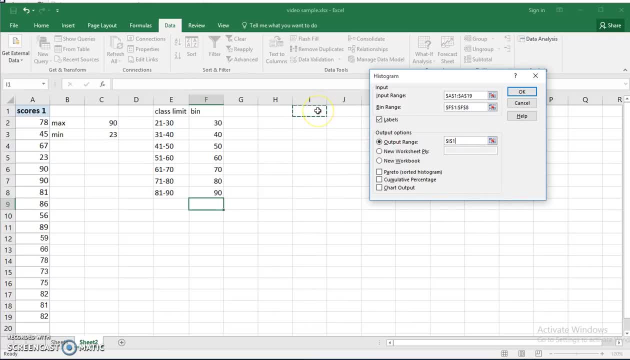 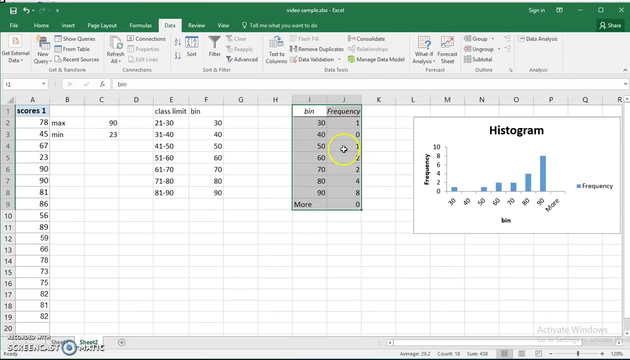 output in this worksheet. so I click a cell in the output range. the last thing I want to do is check output so the histogram would show up, might say: okay, see, I would have. this is the frequency distribution for each class and also this is the histogram. we need to do some adjustment. first of all, we'll copy this. 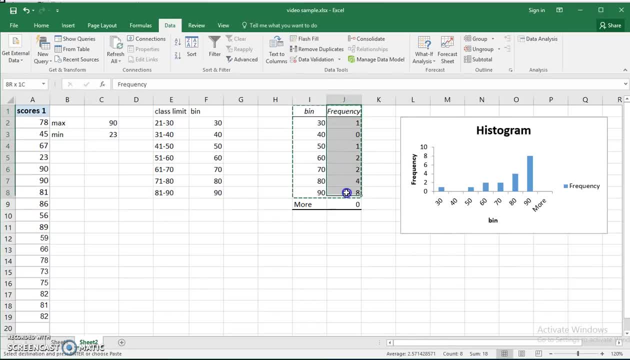 over. well, actually, I just need to copy the frequency over in a new area face and use the what, the class limit that we have set up. so they: this is the class. this is the frequency for this class. there's one data between 21 to 30 and there's a corresponding data values in this range, and that would 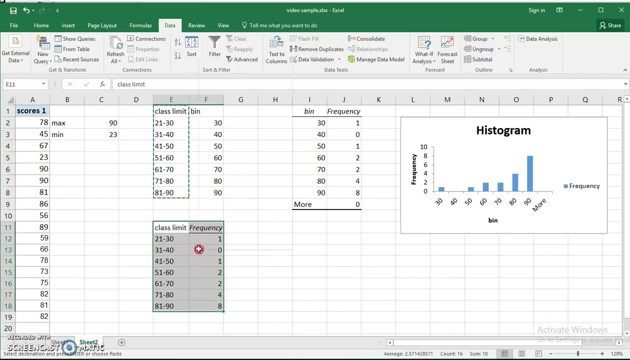 be our frequency distribution and you can, you know, make it nicer by putting in the borders. that's it, and maybe you want to change it not as the class limit, you want to say it as scores for class one, something like that, and then for our histogram, what we can do is change the title, so maybe you will. 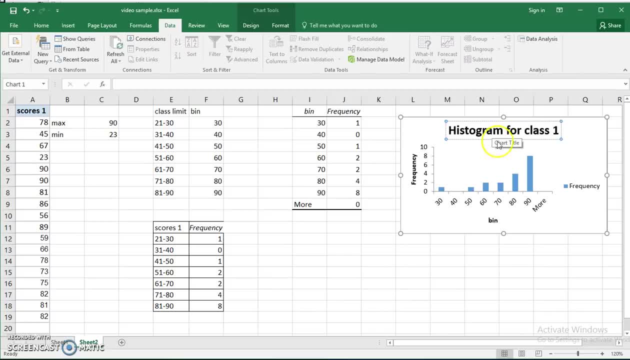 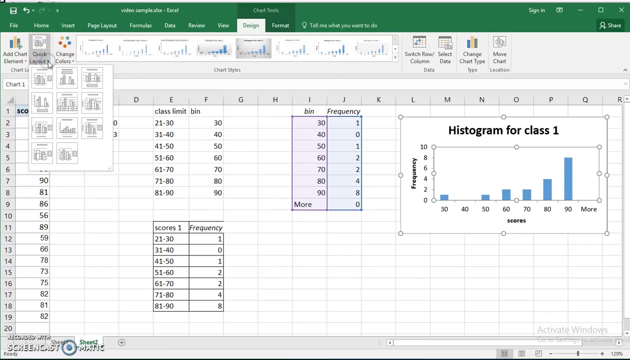 say, histogram for class one: frequency, instead of bin, it should be score right now. delete this. then last thing we want to do is click on the, the, the graph area, click on design. then, under quick layout, I want to choose a layout that that look like a histogram, because histograms not supposed to have space between graph and